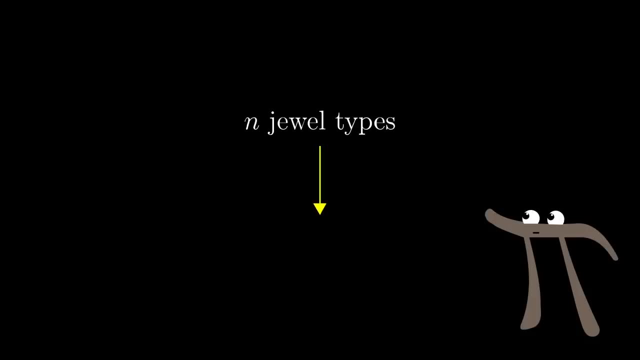 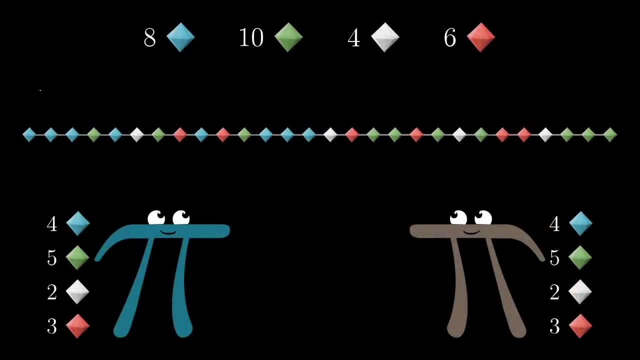 is that if there are N different jewel types, it's always possible to do this fair division with only N cuts or fewer. So with four jewel types in this example, no matter what random ordering of the jewels, it should be possible to cut it in four places and divvy up the five necklace pieces so that 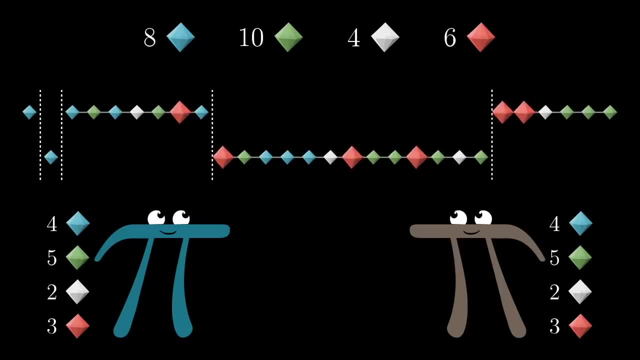 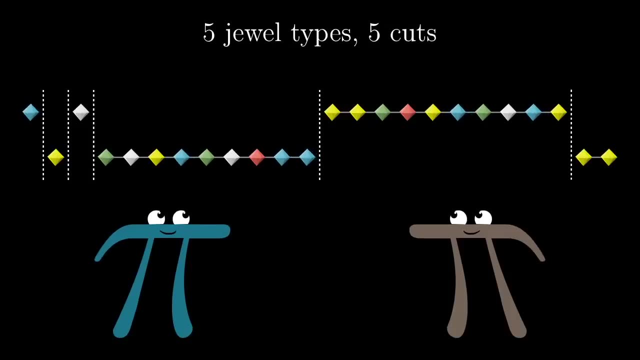 each thief has the same number of each jewel type. With five jewel types, you should be able to do it with five cuts, no matter the arrangement, and so on. It's kind of hard to think about, right? You need to keep track of all of these different jewel types, ensuring 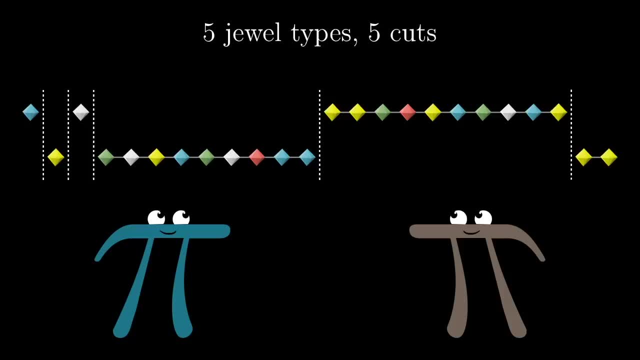 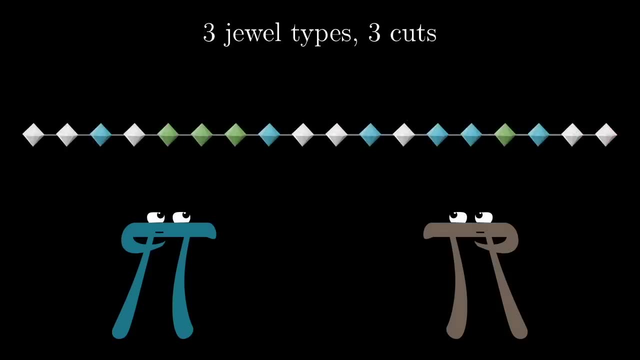 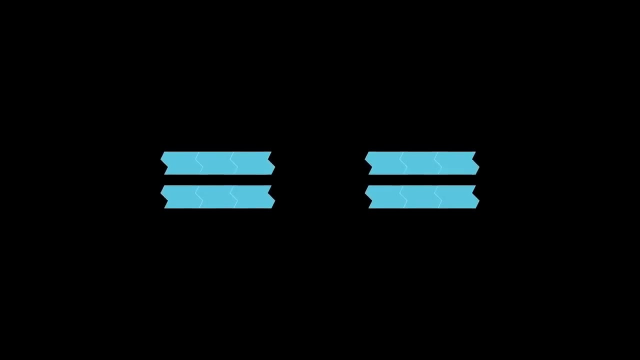 that they're divided fairly while making as few cuts as possible. And if you sit down to try this, this is a shockingly hard fact to prove. Maybe the puzzle seems a little contrived, but its core characteristics like trying to minimize sharding and allocating some collections of things in a balanced way. these are the. 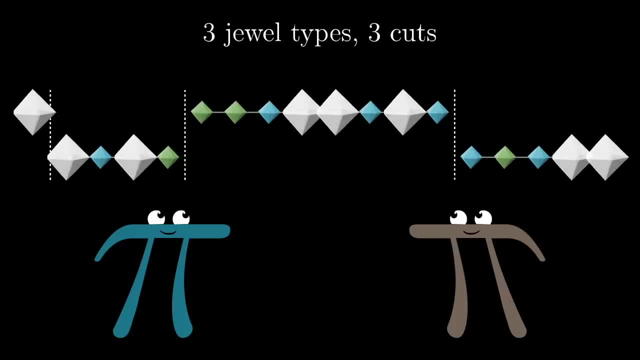 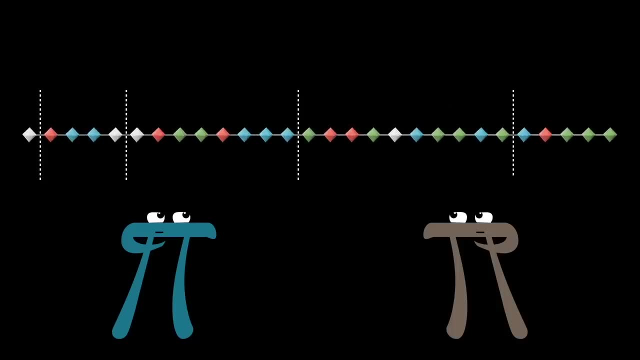 kind of optimization issues that actually come up quite frequently in practical applications. For the computer system folks among you, I'm sure you can imagine how this is analogous to kinds of efficient memory allocation problems. Also for the curious among you, I've left 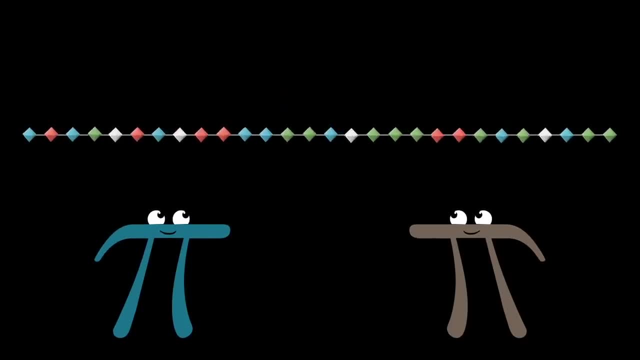 a link in the description to an electrical engineering paper that applies this specific problem. Independent from the usefulness, though, it certainly does make for a good puzzle. Can you always find a fair division using only as many cuts as there are types of jewels? 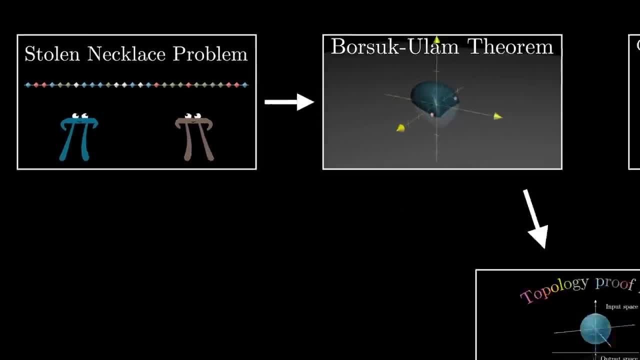 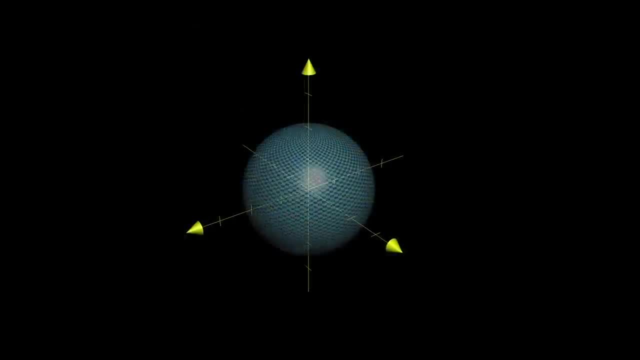 So that's the puzzle, remember it. And now we take a seemingly unrelated sidestep to the total opposite side of the mathematical universe topology. Imagine taking a sphere in 3D space and squishing it somehow onto the 2D plane, stretching and. 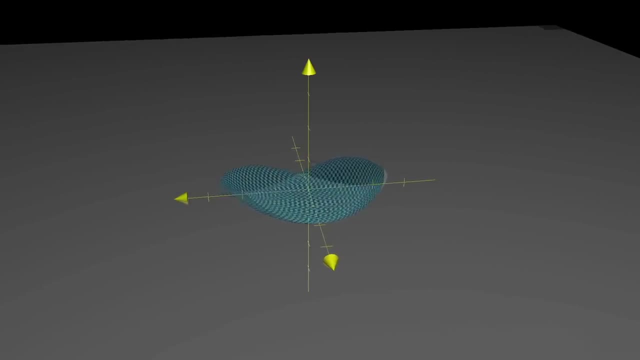 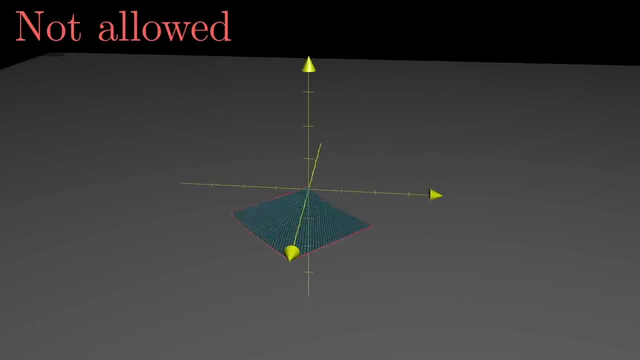 morphing it however you'd like to do so. The only constraint I'll ask is that you do this continuously, which you can think of as meaning never cut the sphere or tear it in any way during this mapping. As you do this, many different pairs of points will 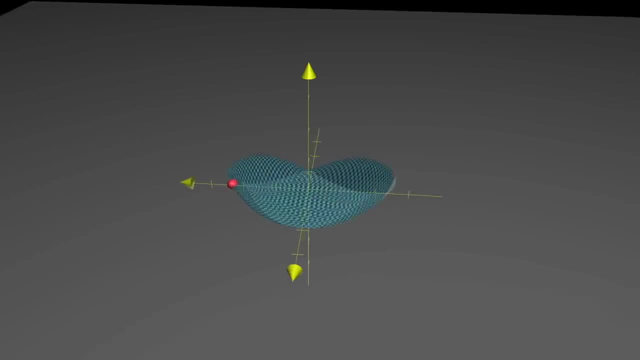 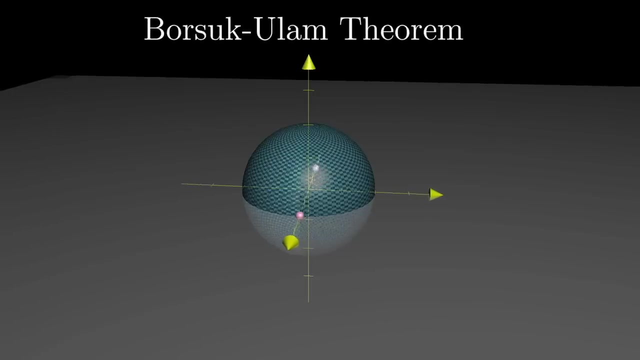 land on top of each other once they hit the plane, and that's not really a big deal. The special fact that we're going to use, known as the Borsuk-Ulam theorem, is that you will always be able to find a pair of points that started off on the exact opposite. 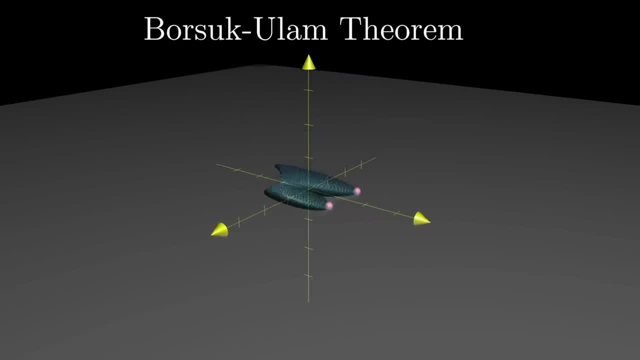 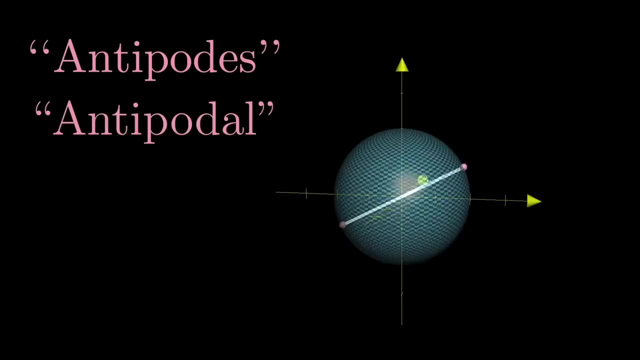 sides of the sphere which land on each other during the mapping Points on the exact opposite, like this, are called antipodes or antipodal points, For example, if you think of the sphere as Earth and you're mapping as a straight projection. 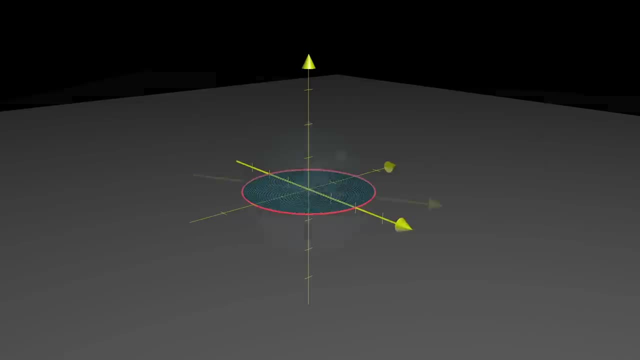 of every point directly onto the plane of the equator, the North and South Pole, which are antipodal, each land on the same point And in this example that's the only antipodal pair that lands on the same point and any other antipodal pair will end up offset from. 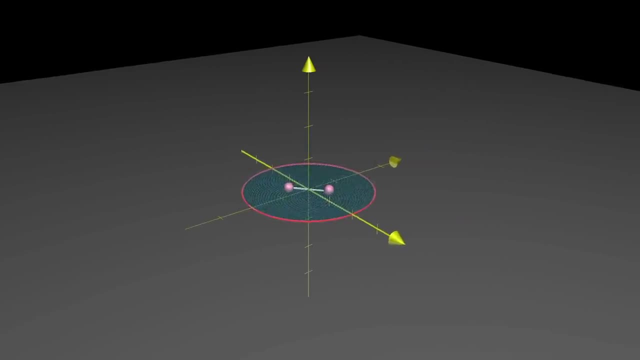 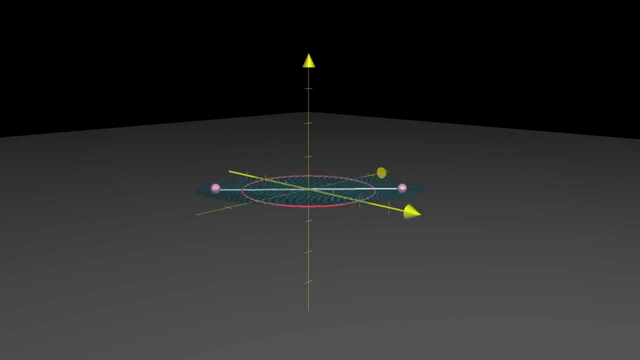 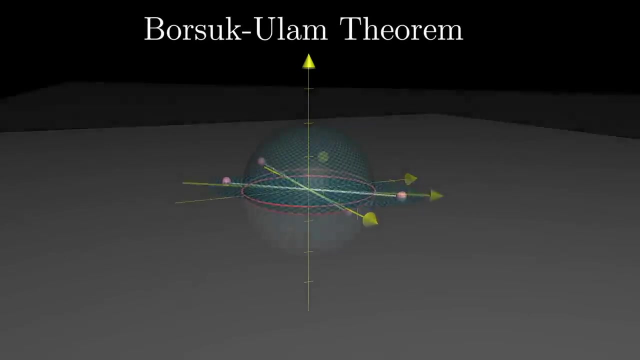 each other. somehow. If you tweaked this function a bit, maybe shearing it during the projection, the North and the South Pole don't land on each other anymore. But when the topology gods close a door, they open a window, because the Borsuk-Ulam theorem guarantees that, no matter what there 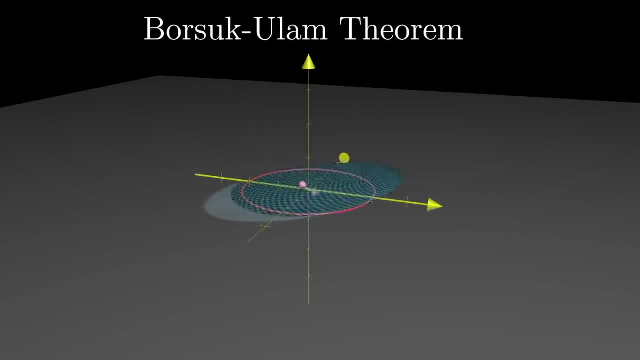 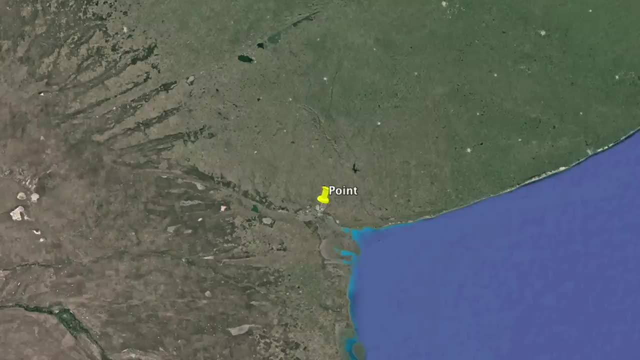 must be some other antipodal pair that now land on top of each other. The classic example to illustrate this idea, which math educators introducing Borsuk-Ulam are required by law to present, is that there must exist some pair of points on the opposite. 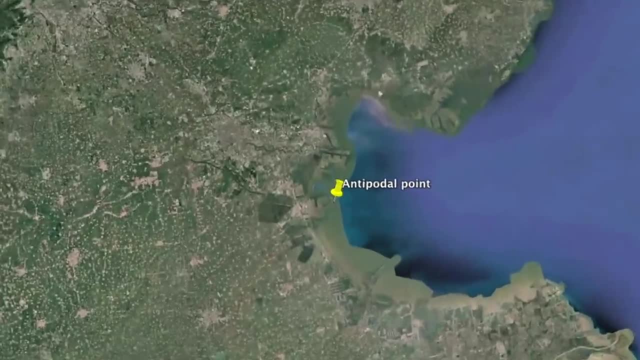 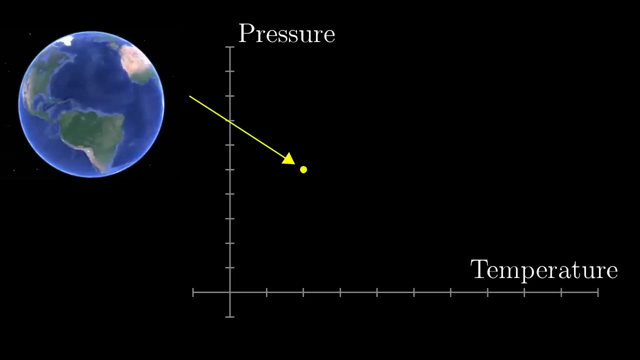 side of the Earth, where the temperature and the barometric pressure are both precisely the same. This is because associating each point on the surface of the Earth with a pair of numbers- temperature and pressure- is the same thing as mapping the surface of the Earth. 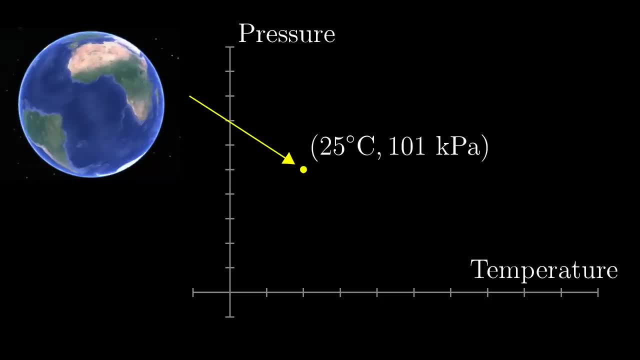 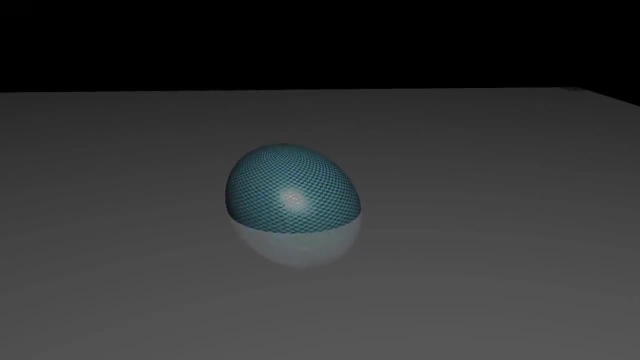 onto a 2D coordinate plane where the first coordinate represents temperature and the second represents pressure. The implicit assumption here is that temperature and pressure each vary continuously as you walk around the Earth. So this association is a continuous mapping from the sphere onto a plane, some non-tearing way to squish that surface into. 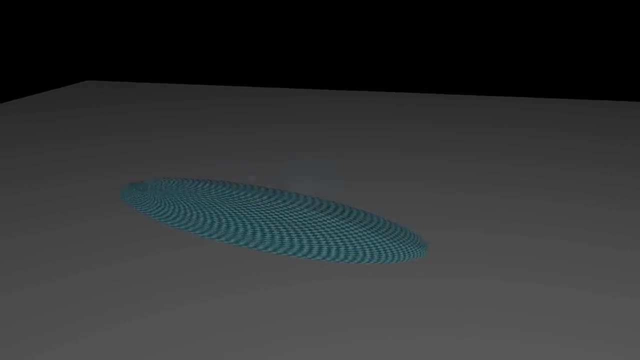 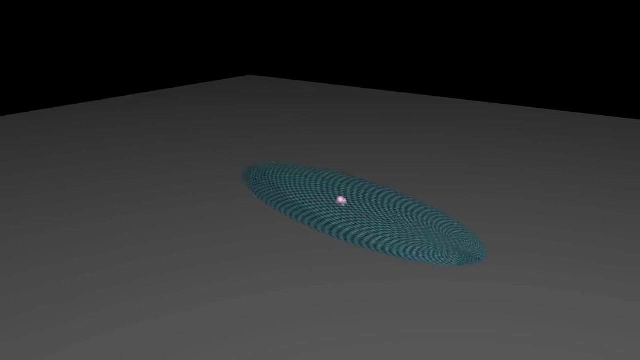 two dimensions. So what Borsuk-Ulam implies is that, no matter what the weather patterns on Earth, or any other planet for that matter, two antipodal points must land on top of each other, which means they map to the same temperature-pressure pair. 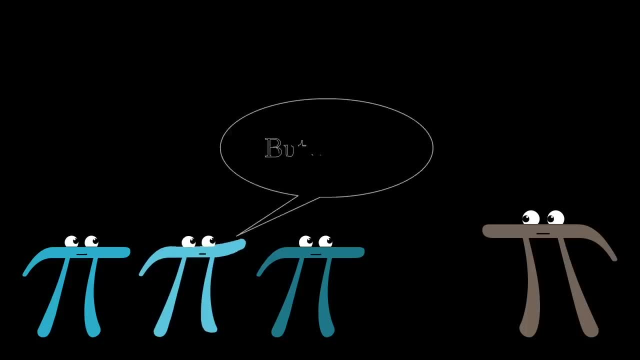 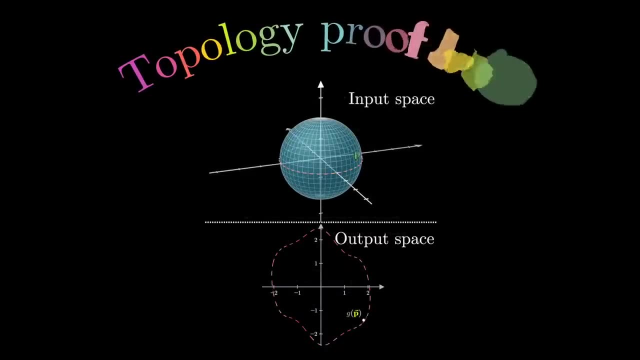 Since you're watching this video, you're probably a mathematician at heart, so you want to see why this is true. not just that, it's true. So let's take a little sidestep through topology-proof land, and I think you'll agree that this is a really 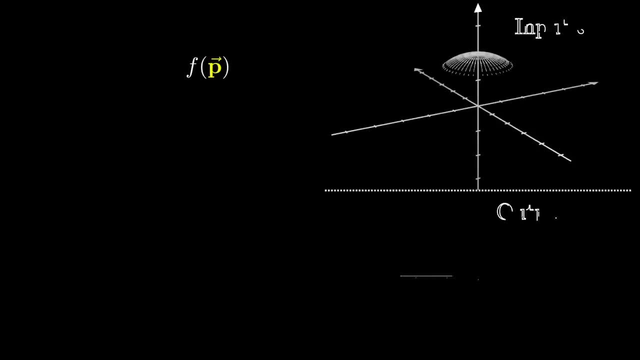 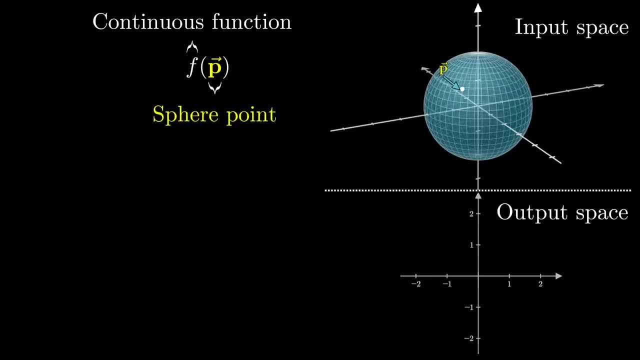 satisfying line of reasoning. First, rephrasing what it is we want to show slightly more symbolically: if you have some function f that takes in a point p of the sphere and spits out some pair of coordinates, you want to show that, no matter what crazy choice of function, this is as long as it's. 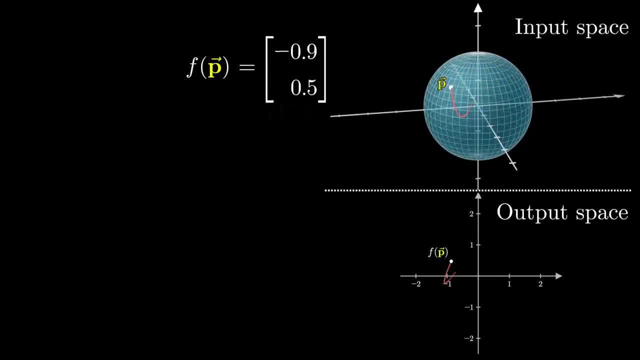 continuous, you'll be able to find some point p, so that f equals f, where negative p is the antipodal point on the other side of the sphere. The key idea here, which might seem small at first, is to rearrange this and say f. 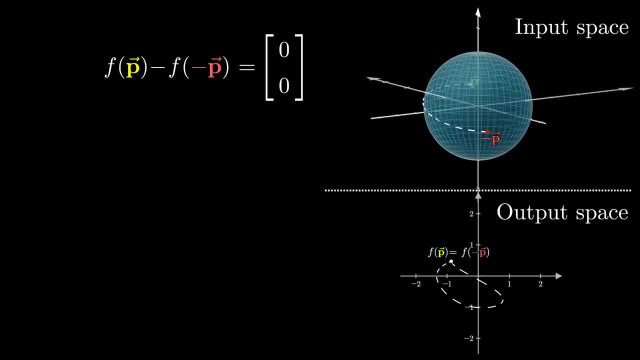 of p minus f of negative p equals 0,0, and focus on a new function, g of p. that's defined to be this left-hand side here: f of p minus f of negative p. This way, what we need to show is that g maps some point of the sphere onto the origin in 2D space. So, rather than 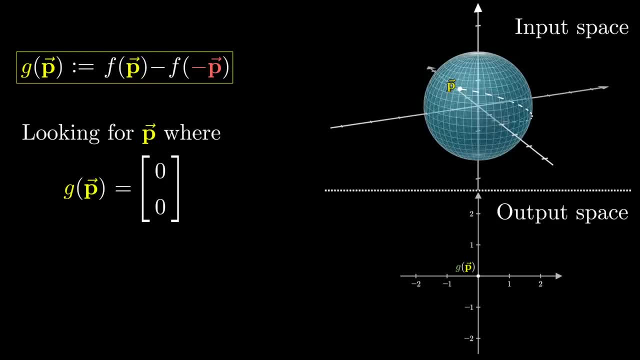 finding a pair of colliding points which could land anywhere. this helps us to find some point p and limit our focus to just one point of the output space: the origin. This function, g, has a pretty special property which will help us out that g of negative. 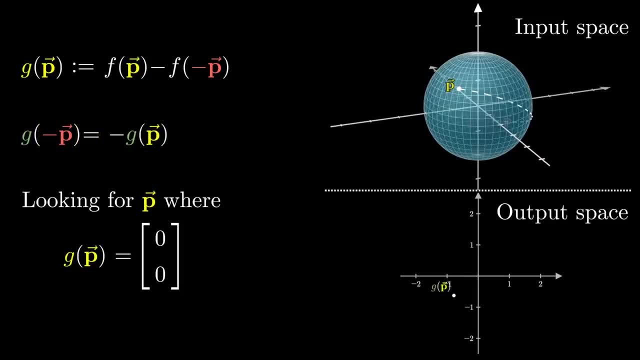 p is equal to negative g of p. Basically, negating the input involves swapping these terms. In other words, going to the antipodal point of the sphere results in reflecting the output of g through the origin of the output space. So you think of it as rotating that output 180 degrees around the origin. 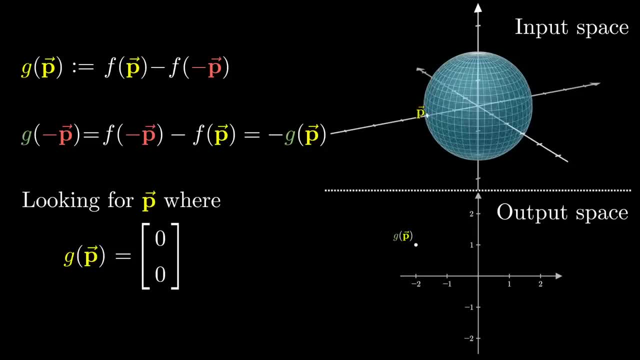 Notice what this means. if you were to continuously walk around the equator and look at the outputs of g, What happens when you go halfway around? Well, the output needs to have wandered to the reflection of the starting point through the origin. Then, as you continue walking around, the other half, the second half of your output path, 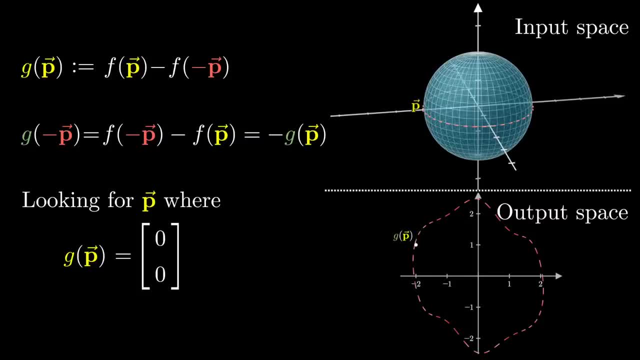 must be the reflection of the first half, Or, equivalently, it's the 180 degree rotation of that first path. Now there's a slim possibility that one of these points happens to pass through the origin, in which case you've lucked out and we're done early. 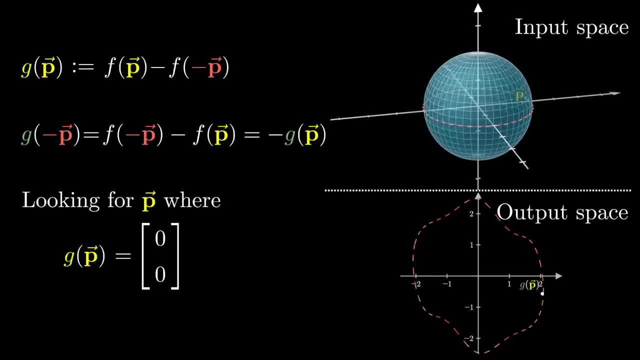 But otherwise what we have here is a path that winds around the origin. at least once Now look at that path on the equator and imagine continuously deforming it up to the north pole, cinching that loop tight. As you do this, the resulting path in the output space is also continuously deforming. 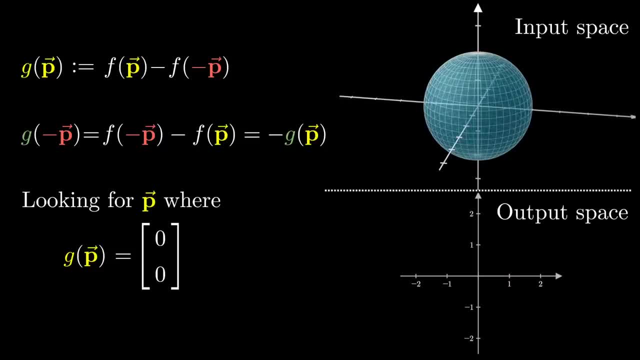 to a point. since the function g is continuous Because it wound around the origin, at some point during this process it must cross the origin and this means there is some point p on the sphere where g has the coordinates, which means f of p minus f of negative p equals, meaning f of p is the 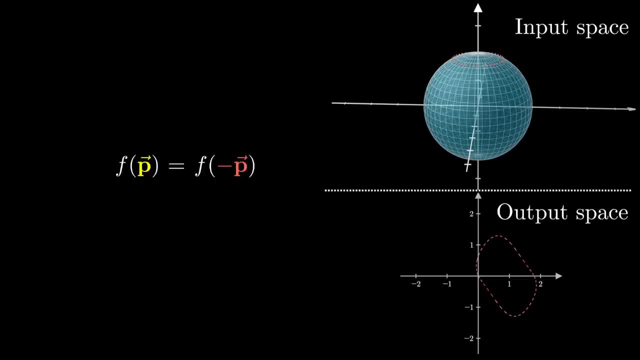 same as f of negative p, the antipodal collision we're looking for. Isn't that clever? And it's a pretty common style of argument in the context of topology. It doesn't matter what particular continuous function from the sphere to the plane, you 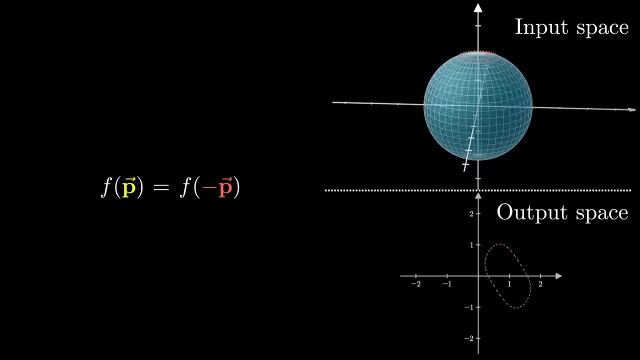 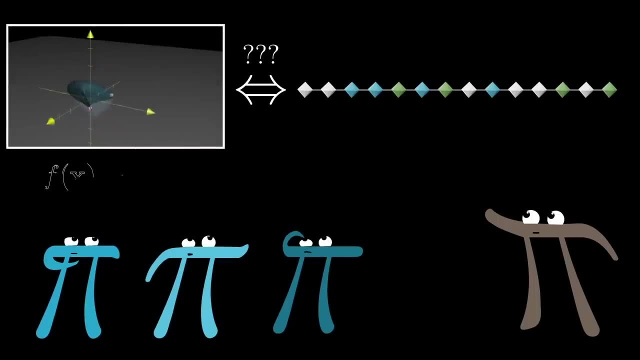 define. this line of reasoning will always zero in on an antipodal pair that lands on top of each other. At this point maybe you're thinking, yeah, yeah, lovely math and all, but we've strayed pretty far away from the necklace problem. 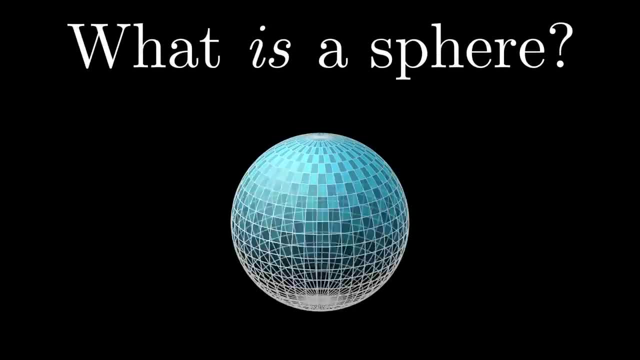 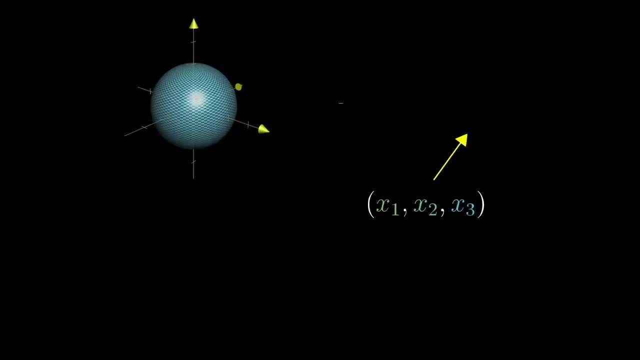 But just you wait. here's where things start getting clever. First answer me this: what IS a sphere really? Well, points in 3D space are represented with 3 coordinates. in some sense, that's what 3D space IS to a mathematician: at least all possible triplets of numbers. 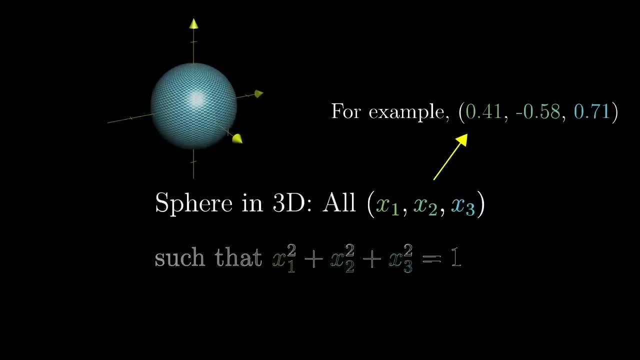 And the simplest sphere to describe with coordinates is the standard unit sphere centered at the origin, the set of all points, a distance one from the origin, meaning all triplets of numbers so that the sum of their squares is one. So the geometric idea of a 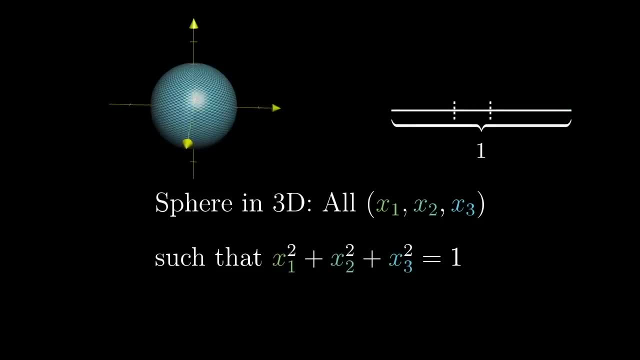 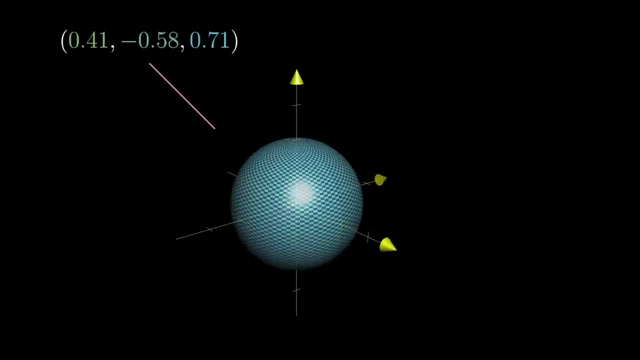 sphere is related to the algebraic idea of a set of positive numbers that add up to one. That might sound simple, but tuck that away in your mind. If you have one of these triplets, the point on the opposite side of the sphere, the corresponding 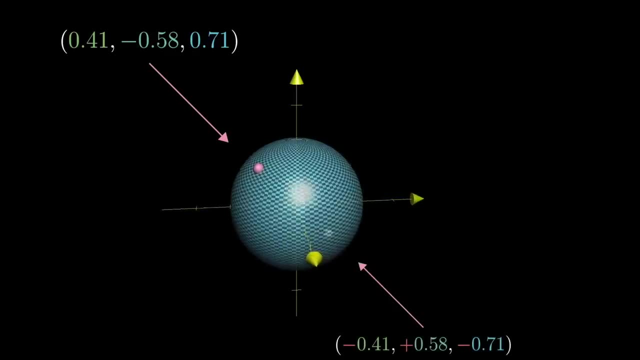 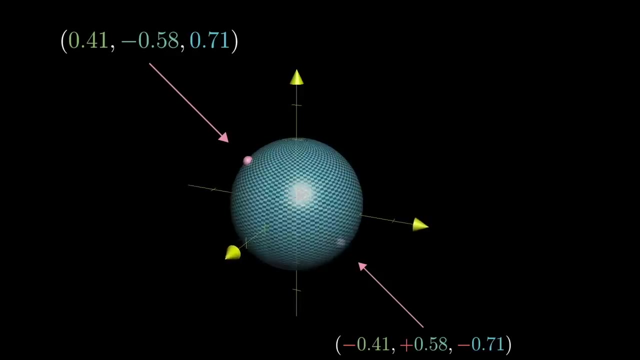 antipodal point is: whatever you get by flipping the sign of each coordinate, right. So let's just write out what the Borsig-Ulan theorem is saying symbolically. Trust me, this will help with getting back to the necklace problem. 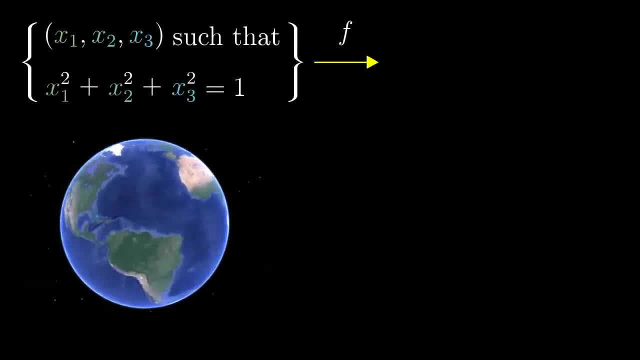 For any function that takes in points on the sphere, triplets of numbers whose squares sum to one, and spits out some point in 2D space, some pair of coordinates like temperature and pressure. as long as the function is continuous, there will be some input, so that flipping 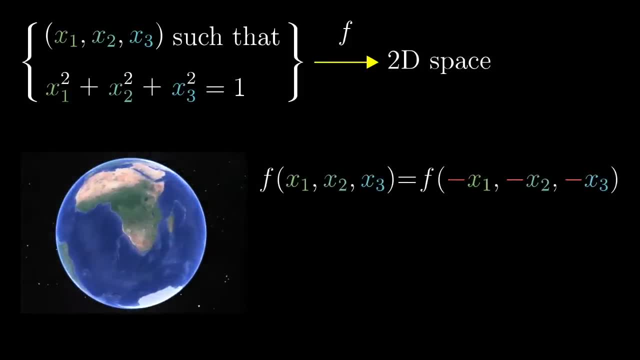 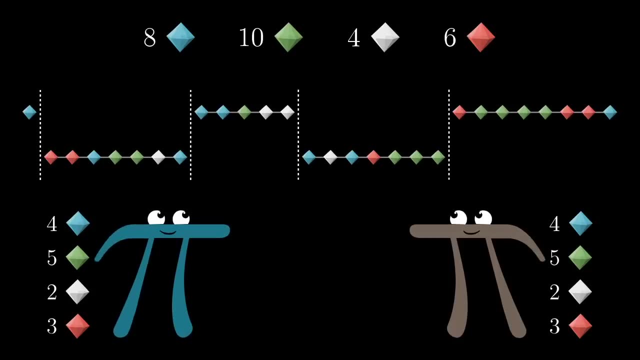 all of its signs doesn't change the output. With that in mind, look back at the necklace problem. Part of the reason these two things feel so very unrelated is that the necklace problem is discrete, while the Borsig-Ulan theorem is continuous. 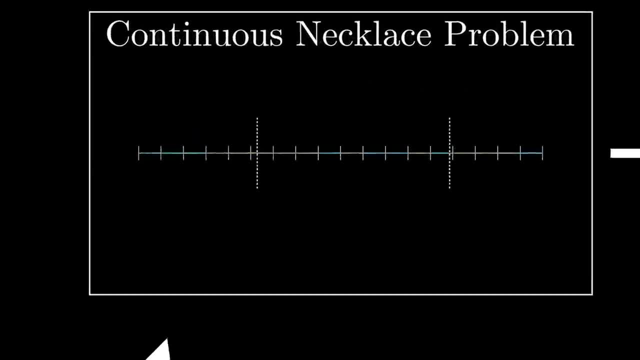 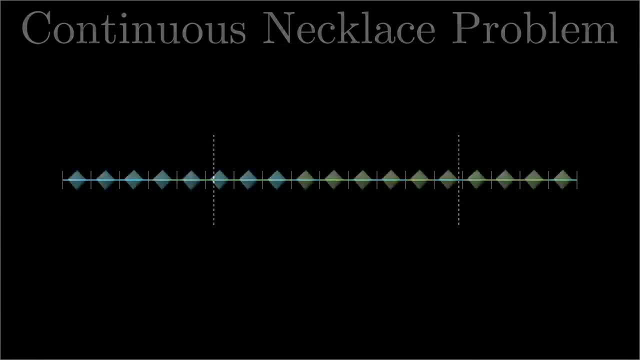 So our first step is to translate the stolen necklace problem into a continuous version. The first step is to find the connection between the necklace divisions and points on the sphere, For right now, let's limit ourselves to the case where there's only two jewel types. 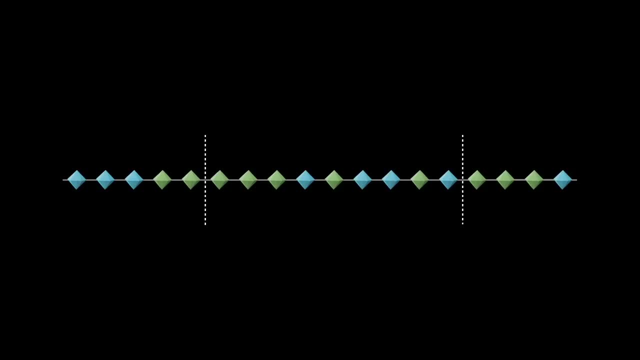 say sapphires and emeralds, and we're hoping to make a fair division of this necklace after only two cuts. As an example, just to have up on the screen, let's say there's 8 sapphires and 10 emeralds. 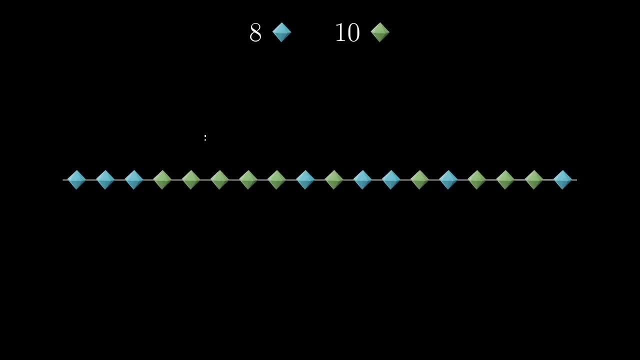 on the necklace, Just as a reminder. this means the goal is to cut the necklace in two different spots and divvy up those three segments so that each thief ends up with half of the necklace. This means that the gold necklace is divided into two parts and the gold necklace is divided. into two parts and the gold necklace is divided into two parts. So the gold necklace is divided into two parts and the gold necklace is divided into two parts. The gold necklace is divided into two parts and the gold necklace is divided into two parts. 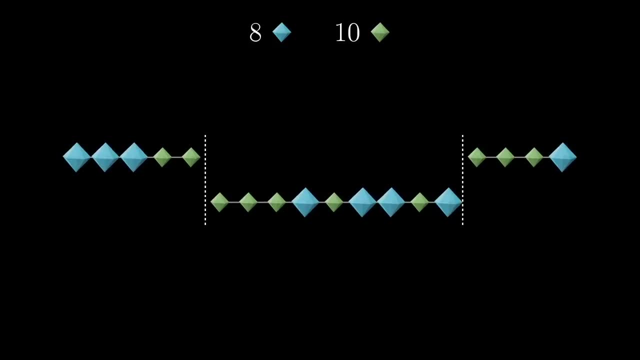 The gold necklace is divided into two parts. and the gold necklace is divided into two parts: Half of the sapphires and half of the emeralds. Notice: the top and the bottom each have 4 sapphires and 5 emeralds. 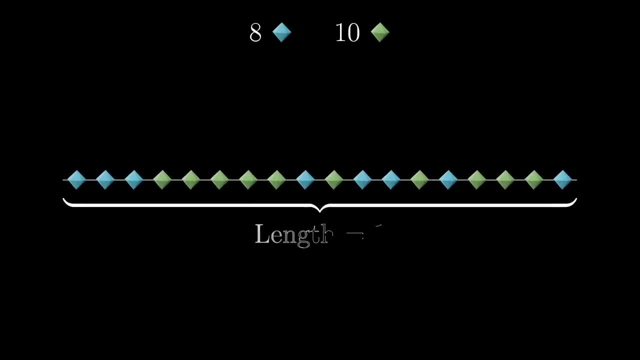 For our continuousification. think of the necklace as a line with length 1, with the jewels sitting evenly spaced on it, and divide up that line into 18 evenly sized segments, one for each jewel, And rather than thinking of each jewel as a discrete, indivisible entity on each segment. 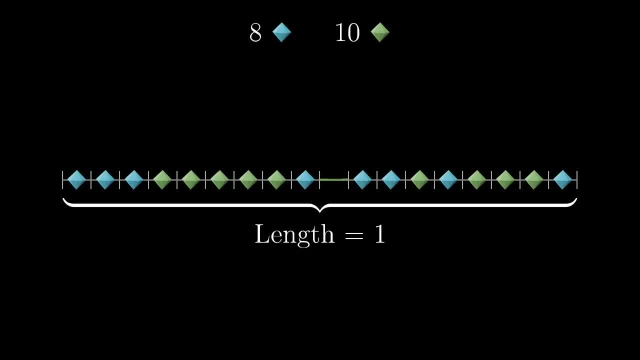 remove the jewel itself and just paint that segment, the color of the jewel. So in this case, 8 eighteenths of the line would be painted sapphire and 10 eighteenths would be painted emerald. The continuous variant of the puzzle is now to ask if we can find two cuts anywhere on. 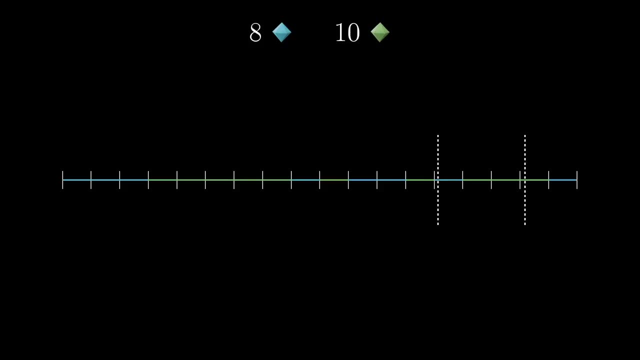 this line, not necessarily on the 1 eighteenth interval marks. that lets us divide up the pieces so that each thief has an equal length of each color. In this case, each thief should have a total of 4 eighteenths of sapphire colored segments. 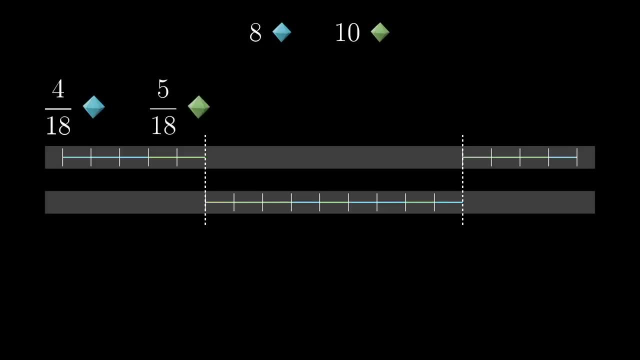 and 5 eighteenths of emerald colored segments. An important but somewhat subtle point here is that if you can solve the continuous variant, you can also solve the original discrete version. To see this, let's say, you did find a fair division whose cuts didn't happen to fall. 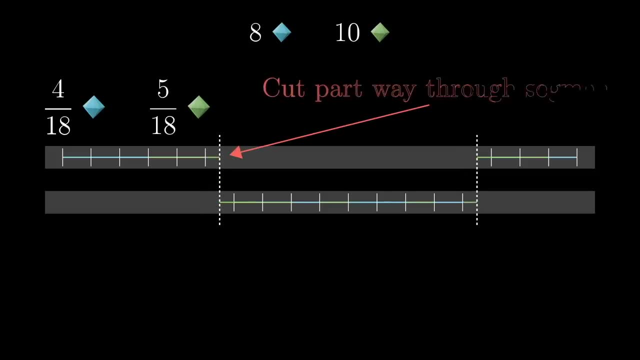 cleanly between the jewels. Maybe it cuts only part way through an emerald segment. Well, because this is a fair division, the length of emerald in both top and bottom has to add up to 5 total emerald segments, A whole number, multiple. 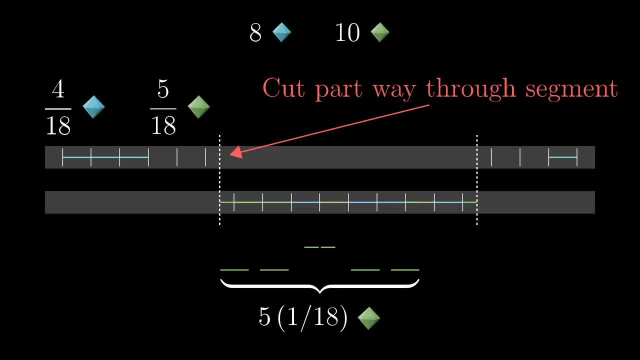 So even if the division cut partially into an emerald segment on the left, it has to cut partially into an emerald segment on the right, and more specifically, in such a way that the total length adds up to a whole number multiple of the segment length. 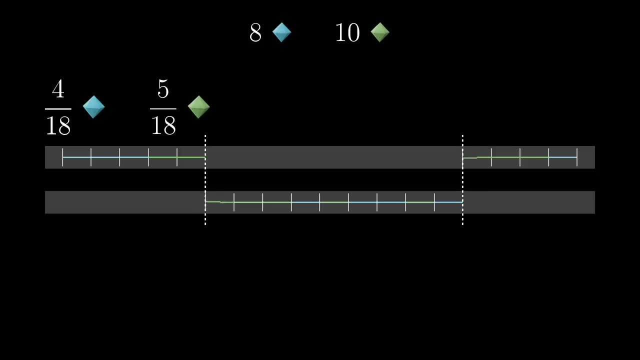 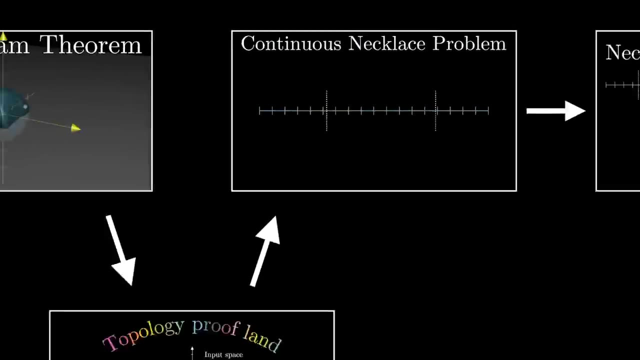 What that means is that you can adjust each cut without affecting the division, so that they ultimately do line up on the 1 eighteenth marks. Now why are we doing all this? Well, in the continuous case where you can cut wherever you want on this line, you can. 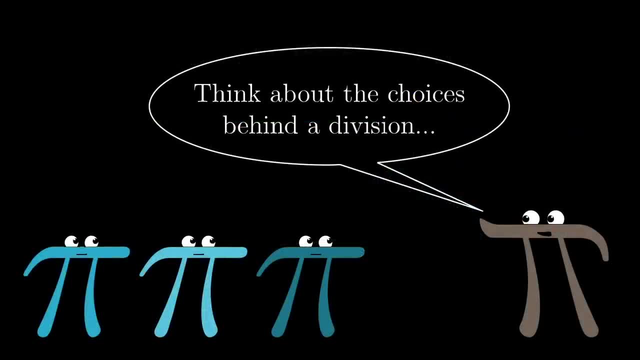 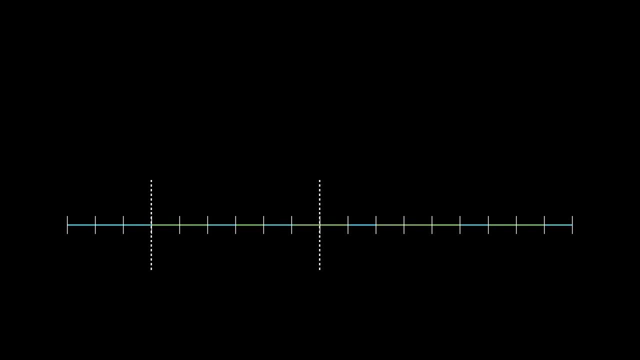 do this. Think about all the choices going into dividing the necklace and allocating the pieces. First, you choose two locations to cut the interval, But another way to think about that is to choose three positive numbers that add up to one. For example, maybe you choose 1 sixth, 1 third and 1 half, which correspond to these. 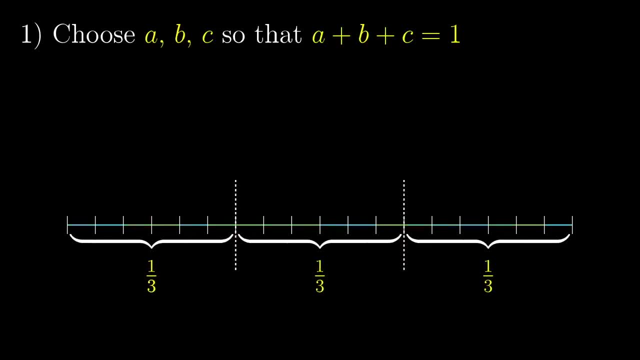 two cuts. Any time you find three positive numbers that add up to one, it gives you a way to cut the necklace and vice versa. After that you have to make a binary choice for each of these pieces. So, for example, if you have a pair of 3 positive numbers, you can cut the necklace with a pair. 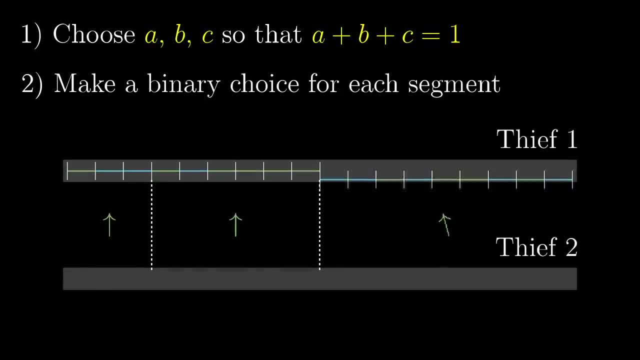 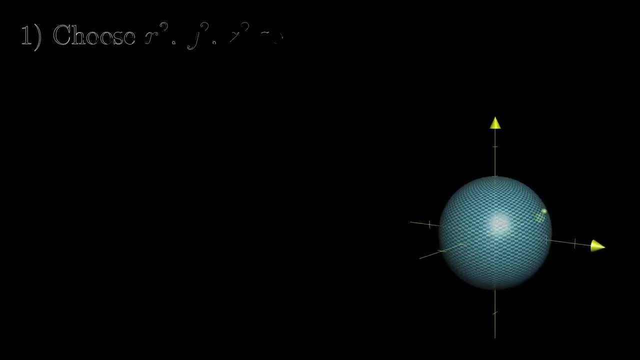 of 3 positive numbers. Now compare that to if I asked you to choose some arbitrary point on a sphere in three dimensional space, Some point with coordinates x, y, z, so that x squared plus y squared plus z squared equals 1.. 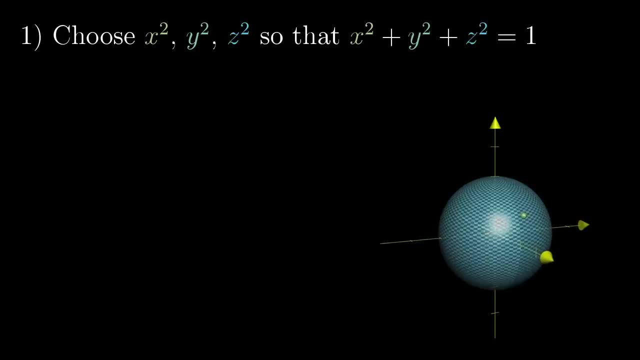 Well, you might start off by choosing three positive numbers that add up to one. Maybe you want x squared to be 1 sixth, y squared to be 1 third and z squared to be 1 half. Then you have to make a binary choice for each one of them, choosing whether to take 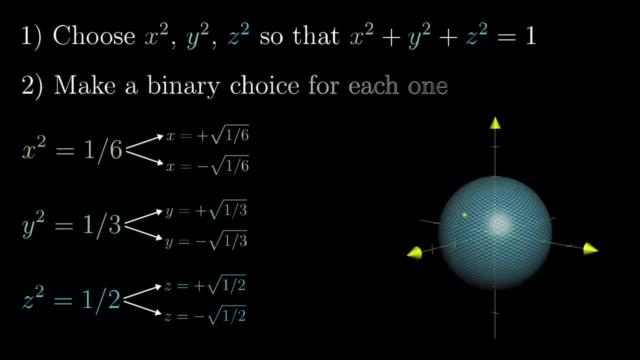 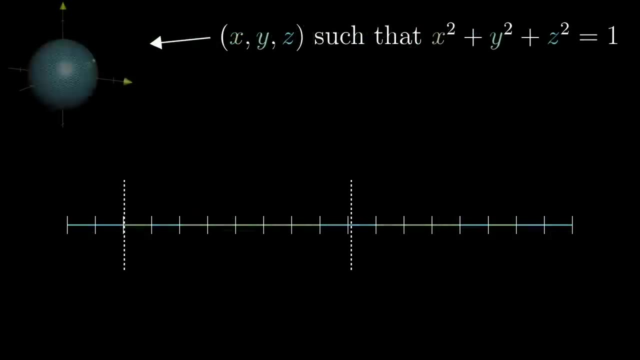 the positive square root or the negative square root, in a way that's completely parallel to dividing the necklace and allocating the pieces. Alright, hang with me now, because this is the key observation of the whole video. It gives a correspondence between points on the sphere and necklace divisions. 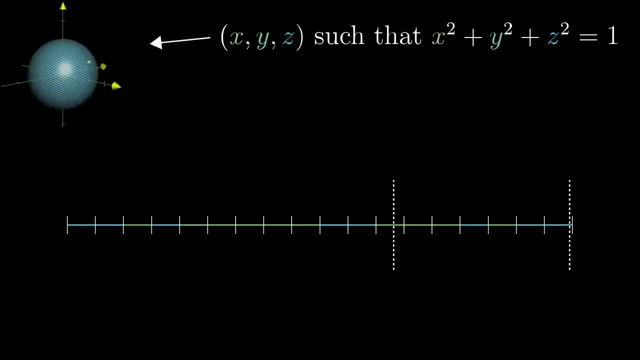 For any point- x, y, z- on the sphere. because x squared plus y squared plus z squared is 1, you can cut the necklace so that the first piece has a length x squared, the second has a length y squared And the third has a length z squared. 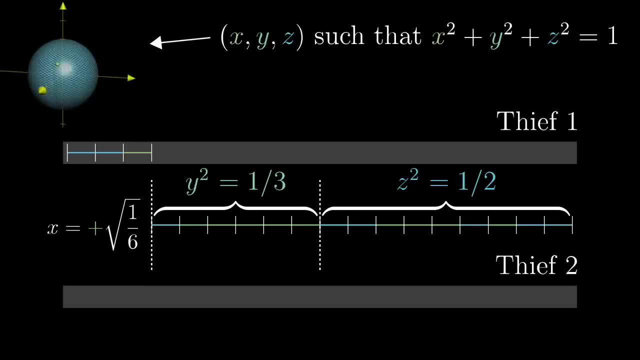 For that first piece, if x is positive, give it to thief 1,, otherwise give it to thief 2.. For the second piece, if y is positive, give it to thief 1, otherwise give it to thief 2.. And likewise, give the third piece to thief 1 if z is positive and to thief 2 if z is. 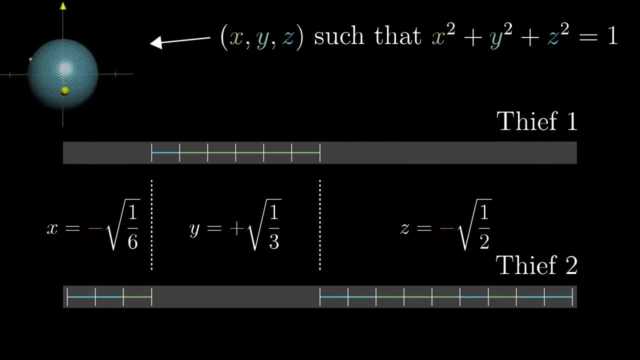 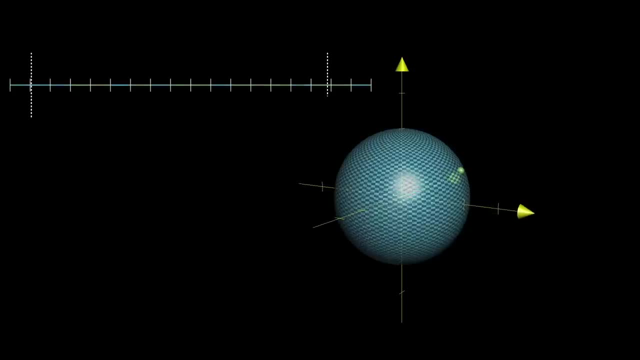 negative, And you could go the other way around. Any way that you divide up the necklace and divvy up the pieces gives us a unique point on the sphere. It's as if the sphere is a weirdly perfect way to encapsulate the idea that the sphere 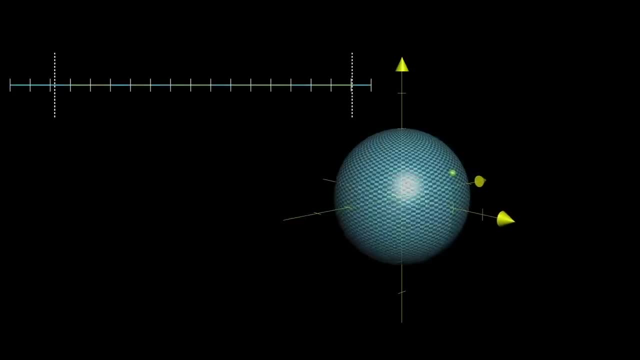 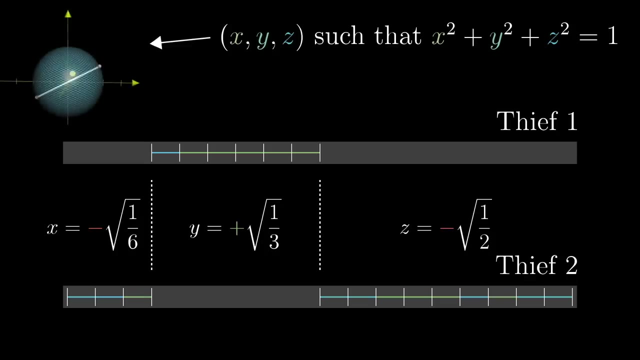 is a point on the sphere. It's as if the world was made of all kinds of Nagra-like objects. And here we are tantalizingly close. Think of the meaning of antipodal points under this association. If the point x, y, z on the sphere corresponds to some necklace allocation, what does the 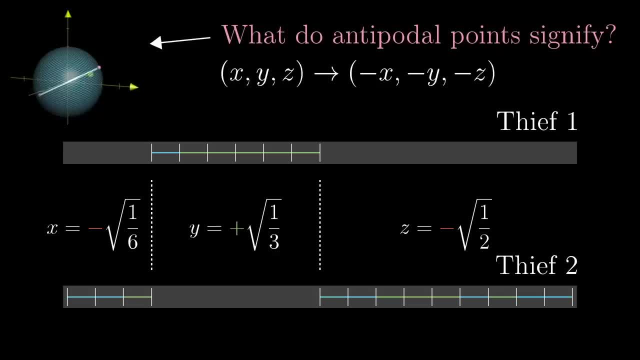 point. negative x, negative y and negative z correspond to. Well, the squares of these three coordinates are the same, so each one corresponds to making the same cut on the necklace. The difference is that every piece switches and changes which is which thief it belongs to. 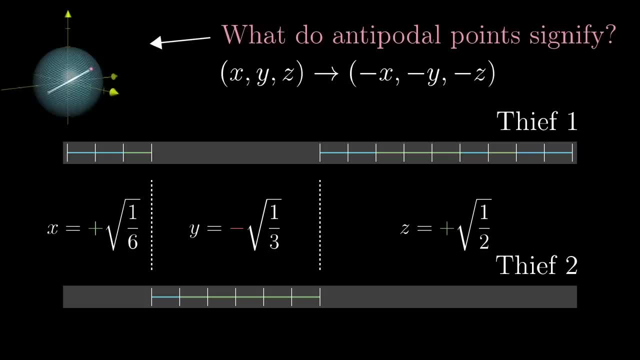 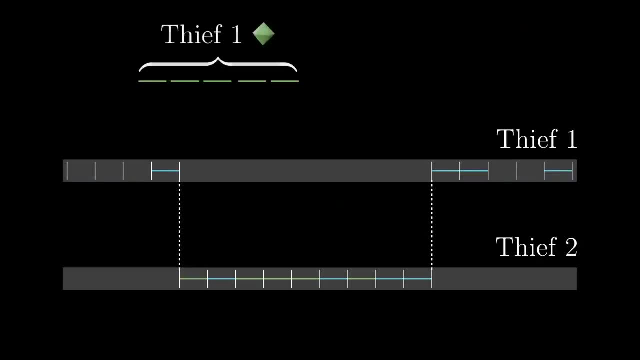 So jumping to an antipodal point on the opposite side of the sphere corresponds with exchanging the pieces. Now remember what it is that we're actually looking for. We want the total length of each jewel type belonging to thief 1 to equal that for thief. 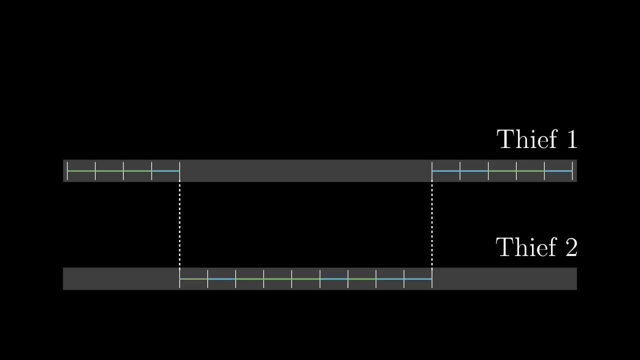 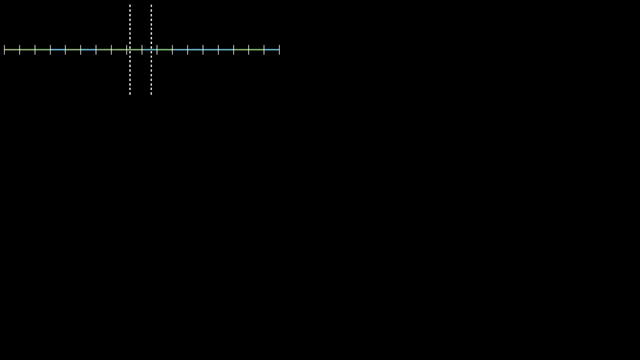 2. Or in other words, in a fair division. performing this antipodal swap doesn't change the amount of each jewel belonging to each thief. Your brain should be burning with the thought of Borsuk Ulam at this point. Specifically, you might construct a function that takes in a given necklace allocation. 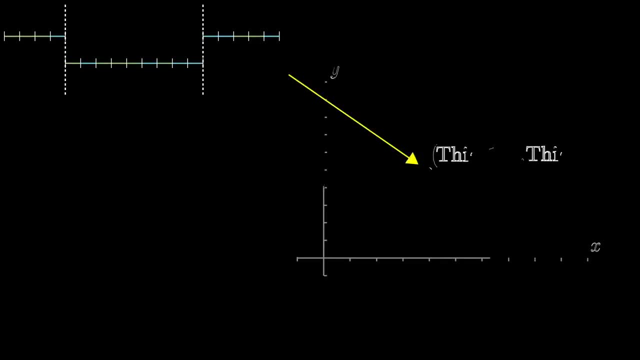 and spits out two numbers: the total length of sapphire belonging to thief 1, and the total length of emerald belonging to thief 1.. We want to show that there must exist a way to divide the necklace with two cuts and divvy. 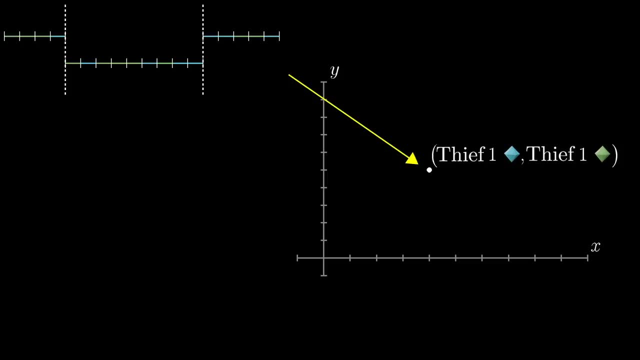 up the pieces so that these two numbers are the same as what they would be for thief 2.. Or said differently, where swapping all of the pieces would be the same as what they would be for thief 2.. Or said differently, where swapping all of the pieces would be the same as what they would be for thief 2.. 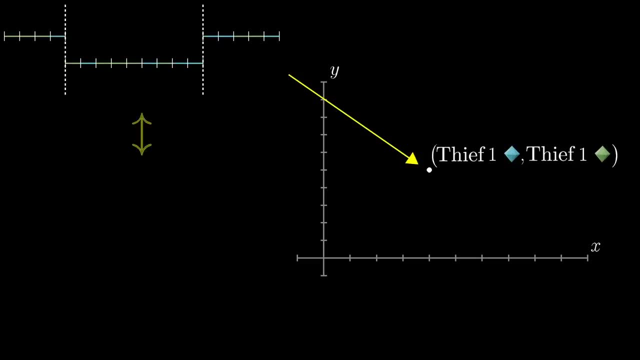 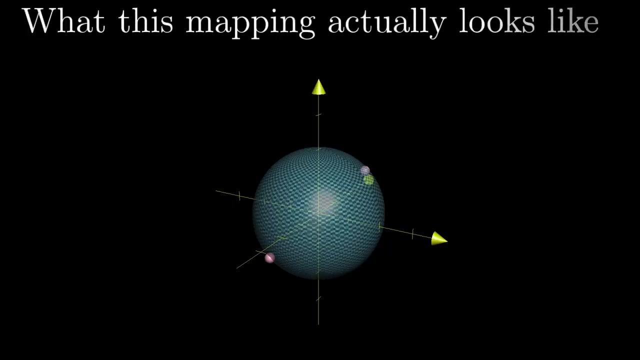 Because of this back-and-forth between necklace allocations and the points of the sphere, and because pairs of numbers correspond with points on the xy-plane, this is in effect a map from the sphere onto the plane, And the animation you're looking at now is that literal map for the necklace. I was 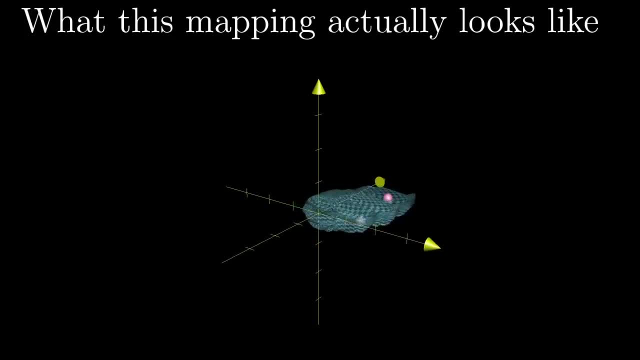 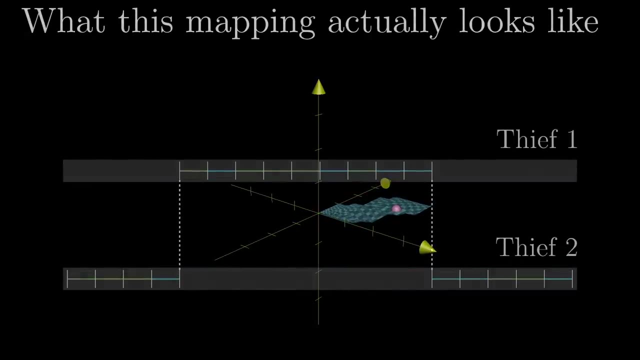 showing. So the Borsuk Ulam theorem guarantees that some antipodal pair of points on the xy-plane, the sphere, land on each other in the plane, which means there must be some necklace division using two cuts. that gives a fair division between the thieves. 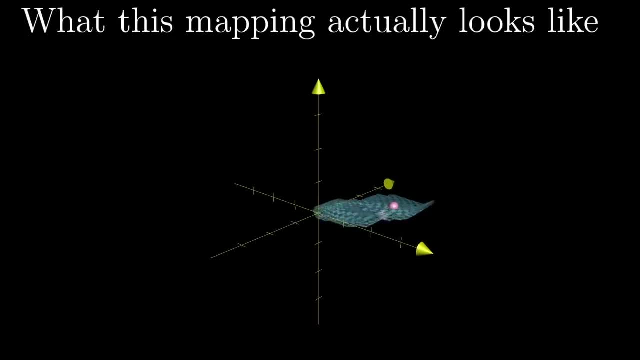 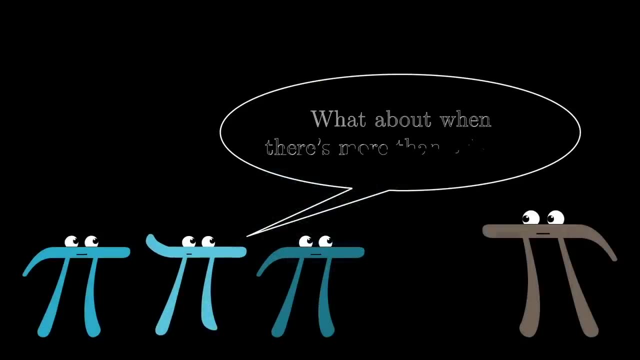 That, my friends, is what beautiful math feels like. Alright, and if you're anything like me, you're just basking in the glow of what a clever proof that is, and it might be easy to forget that what we actually want to solve is the. 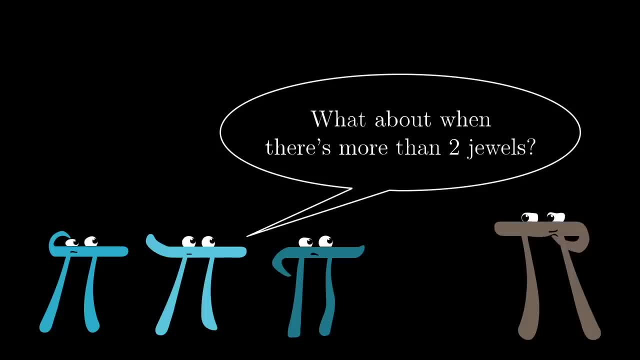 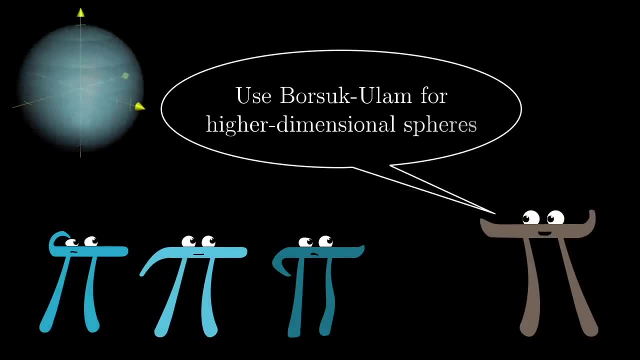 more general stolen necklace problem with any number of jewel types. Luckily, we've now done 95% of the work. generalizing is pretty brief. The main thing to mention is that there is a more general version of the Borsuk-Ulam. 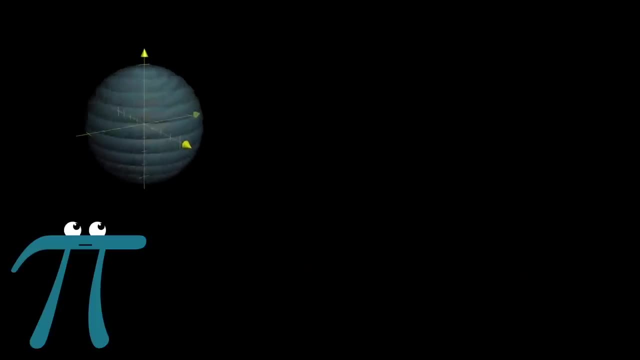 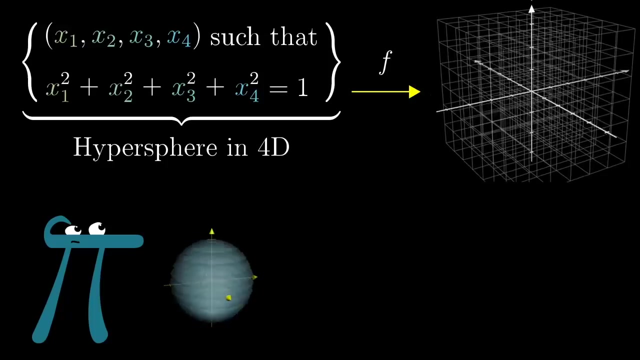 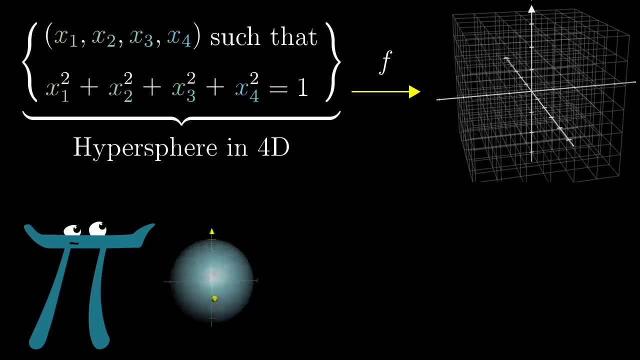 theorem, one that applies to higher-dimensional spheres. As an example, Borsuk-Ulam applies to mapping hyperspheres in 40-space into three dimensions, And what I mean by a hypersphere is the set of all possible lists of four coordinates where the sum of their squares equals 1.. 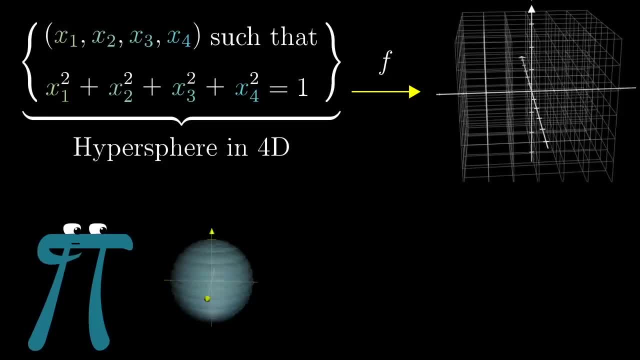 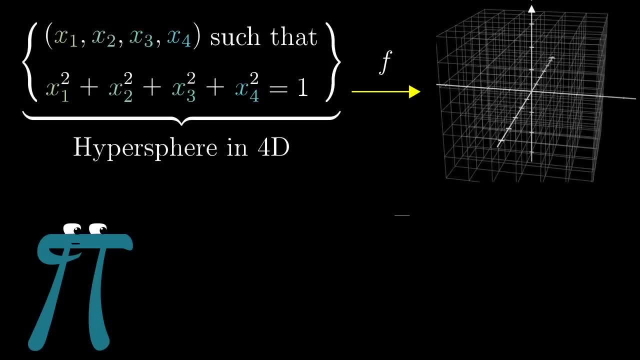 Those are the points in 40-space a distance 1 from the origin. Okay, Okay, Borsuk-Ulam says that if you try to map that set all those special quadruplets of numbers into three-dimensional space, continuously associating each one with some triplet of, 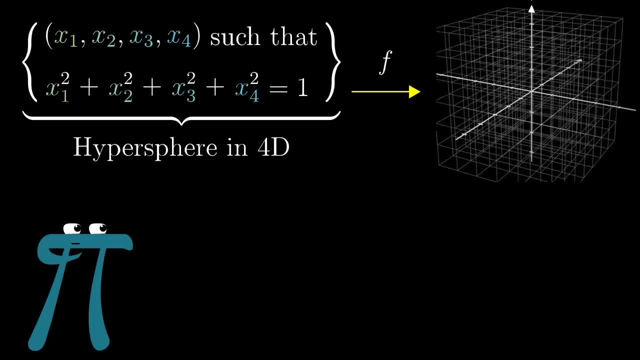 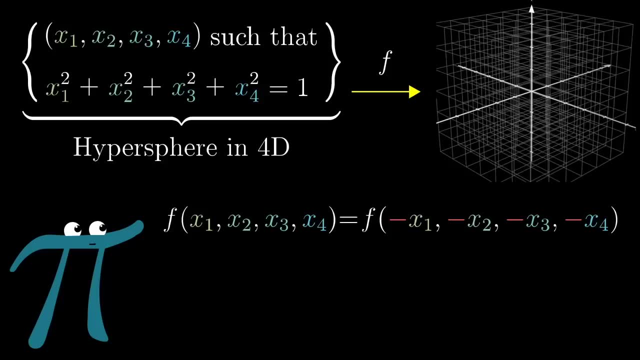 numbers. there must be some antipodal collision, an input x1, x2,, x3, x4, where flipping all of the signs wouldn't change the output. I'll leave it to you to pause and ponder and think about how this could apply to the. 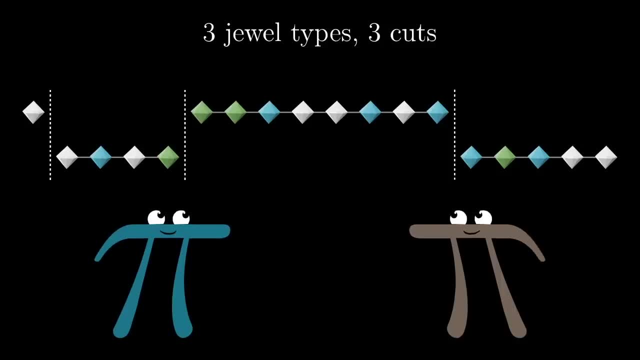 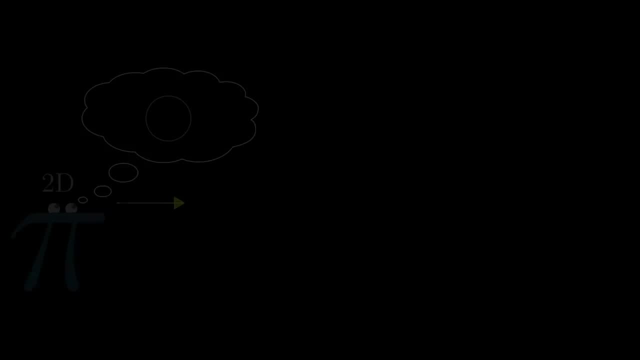 three-jewel case and about what the general statement of Borsuk-Ulam might be and how it applies to the general necklace problem. And maybe, just maybe, this gives you an inkling of why mathematicians care about things like.